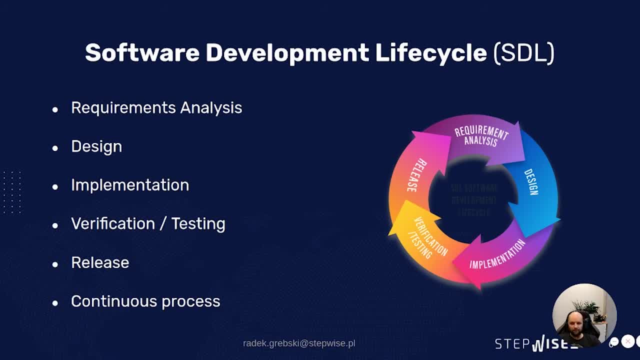 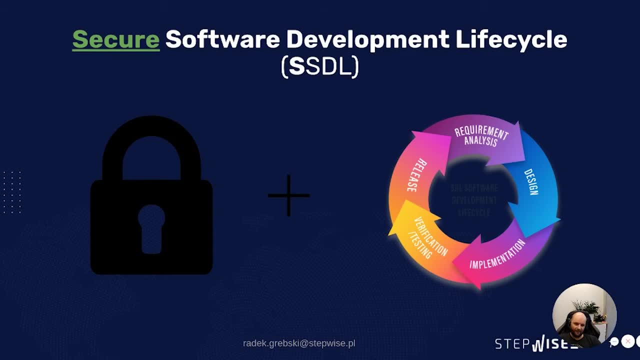 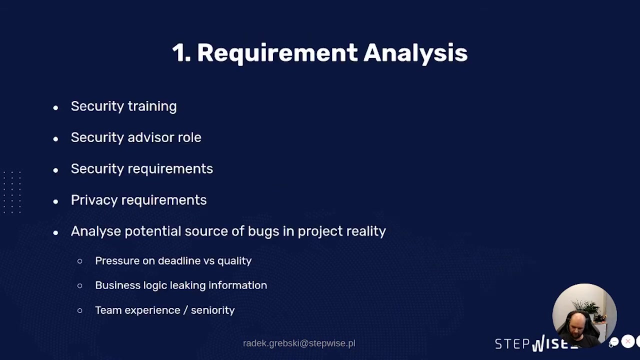 It can be even multiple times a day. So how can we make our software development life cycle secure? We simply add a different security aspects, a different stages of software development life cycle. So let's start with requirement analysis. At this point, our goal should be to make our developers 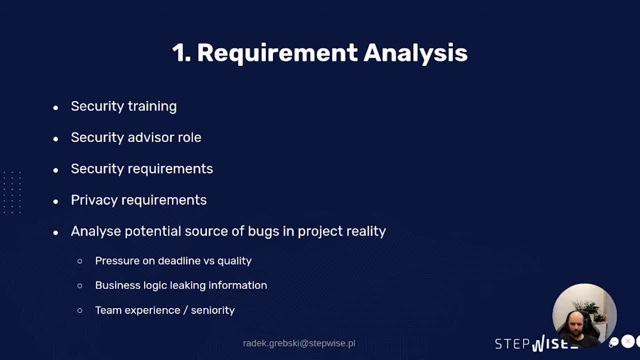 to make the whole team aware about security aspects. So what we can do, we can do security training. It can be done internally if we have a person that is experienced and aware of security aspects. We should also create or assign someone security advisor role. 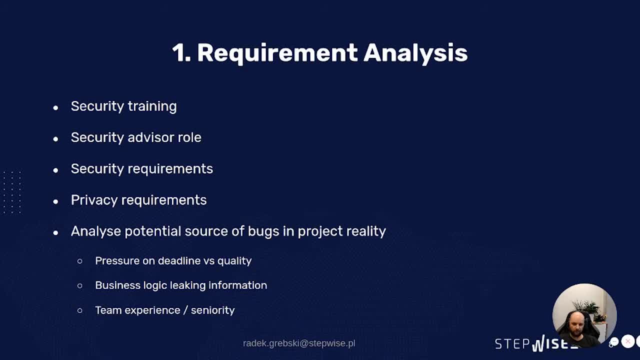 There should be a person or a team responsible for taking care of security aspects of our application. We should also collect security requirements of our application, not only the business ones. We should also think about privacy requirements, For example. GDPR puts a lot of pressure on that. 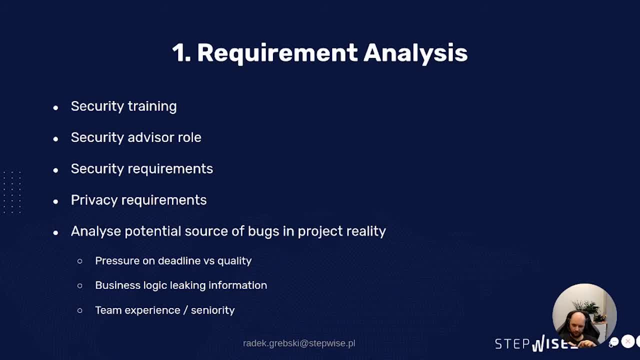 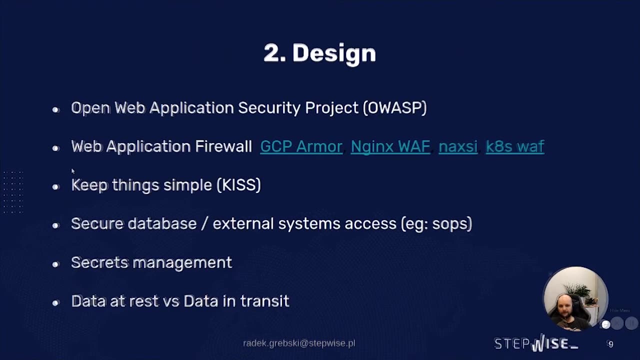 So this is something we should also consider And we should analyze potential sorts of bugs in our project reality. This can be pressure on deadlines, Business logic. that can be leaking information, Our team experience. So, once we deal with security aspects, R and PCI, 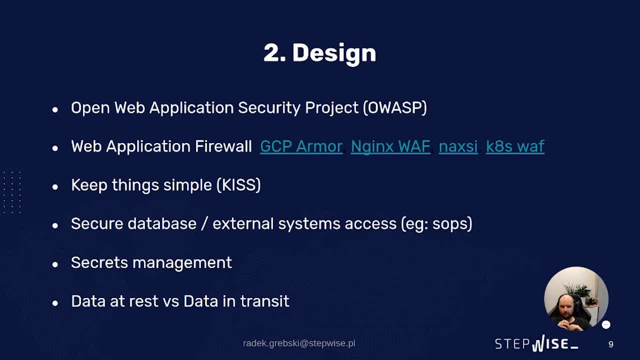 deal with requirement analysis, we go to design phase. at this point, when we are designing the application, there is a very valuable project called open web application security project, which i will talk a bit more on next slides. we can take advantage of web application firewall that protects us from various threats. we should keep things simple, because the more complex, the 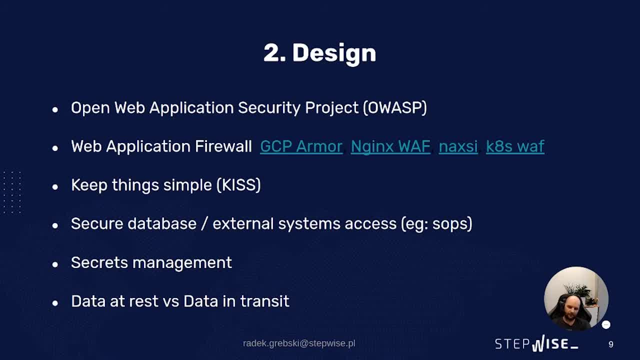 system or is the? there is a bigger chance of making mistake or leak the data. we should also secure database and other external systems access. if we are storing, for example, credentials, we shouldn't store them in a plain text. we can use tools like sops. i will also show it in in the next slides. 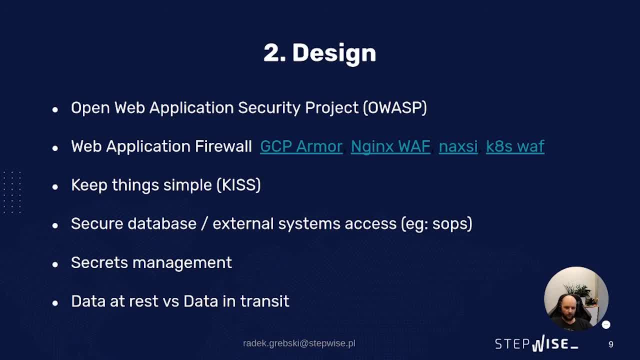 we should also think about secret management at this point: how we gonna store and use secrets. who has access to secrets, where they are stored? either it's going to be kubernetes secrets- if that's the case, who has access to that? and we should also care about data at rest and data in. 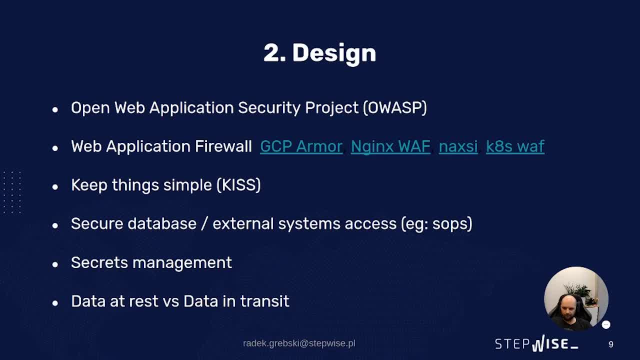 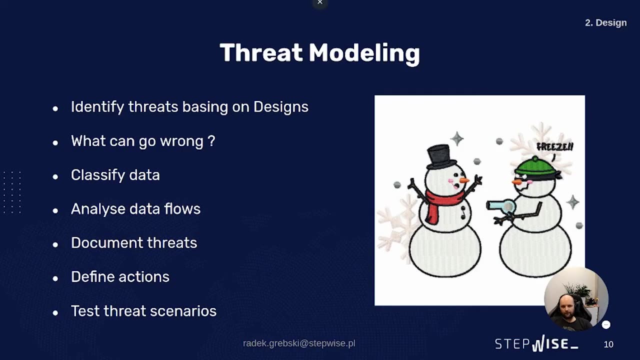 transit, for example, data in transit, we can use ssl and at a data at rest. i mean stuff like backups and stuff that should be encrypted, and we should think about it at early stage, which is design phase. okay, what's also important at design stage is threat modeling. we should identify threads. 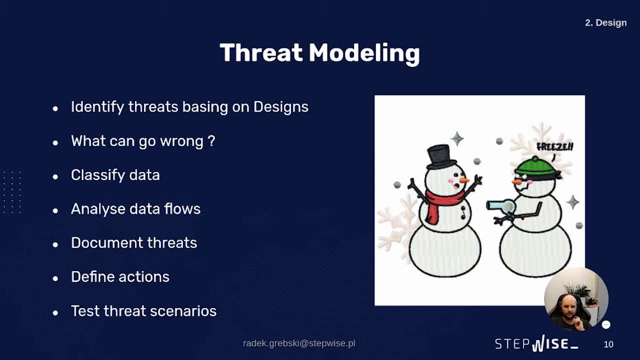 basing on designs. we should think about what can go wrong in our system. we should classify the data. for example, if we store like first names, last names, this stuff is going to be more protected and should. we should put more attention to that rather than, for example, if we collect logs, ip addresses. it's not that. 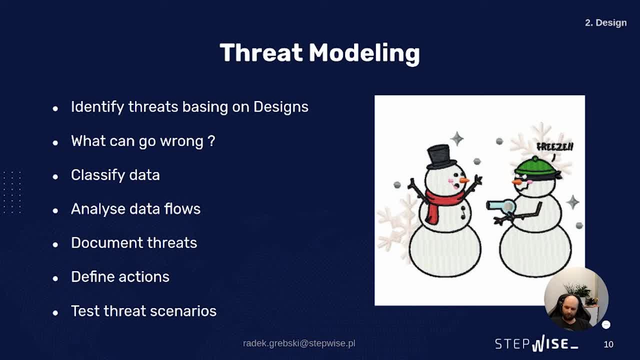 even though with ip addresses also gdpr affected because it's a, it's a treated as a personal data. but it's not that important to to to protect the ip address like we want to protect the first name, last name, id number and stuff like that. we should also analyze the data flows to find. 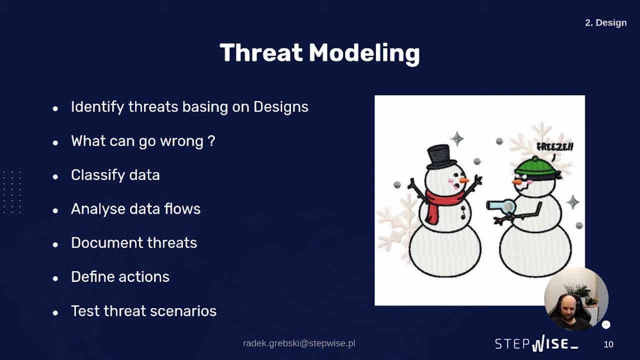 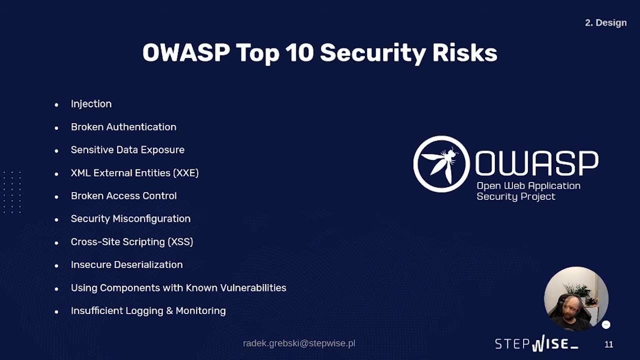 any colliding flows or flows that can leak the data, and once we identify threats, which we should document them, and after that we should define actions and test those threat scenarios. so what can be useful at design stage as well is open web application security projects. there is. 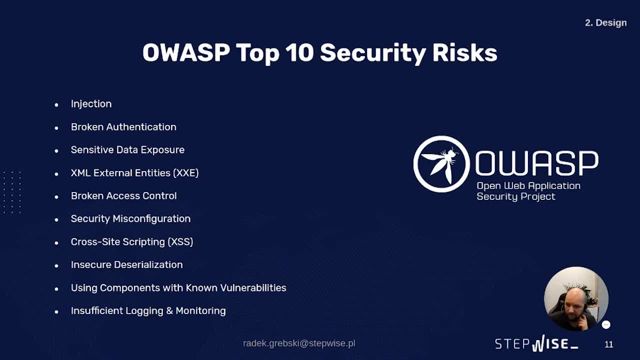 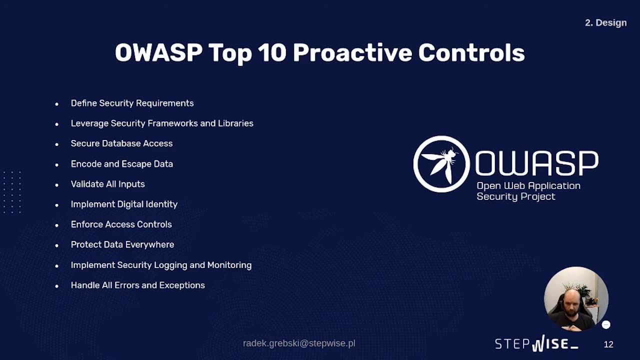 there there is top 10 security risks that i believe every developer should be familiar with, and here you can see the list of those risks. you can also see the top 10 proactive controls that you can do to minimize the risk. so this is like a like a short information on on top security risk and top proactive controls, but what's more? 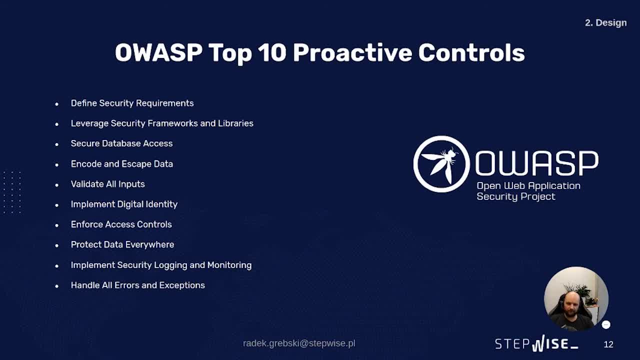 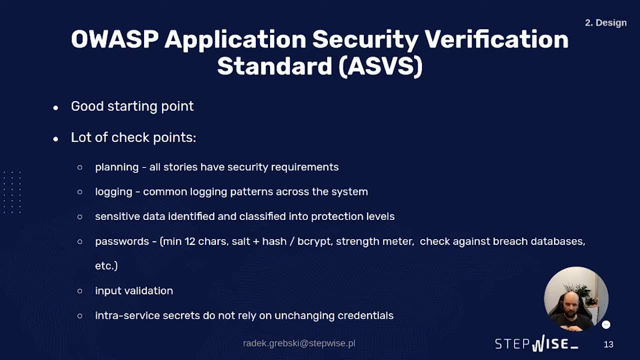 valuable on that project is application security verification standard. this is a very, very good starting point because it has a lot of checkpoints. if you want to build your own security verification standard or software development life cycle, this should be a starting point, because i just noted couple of interesting checkpoints from that document, which is, for example, during the planning all 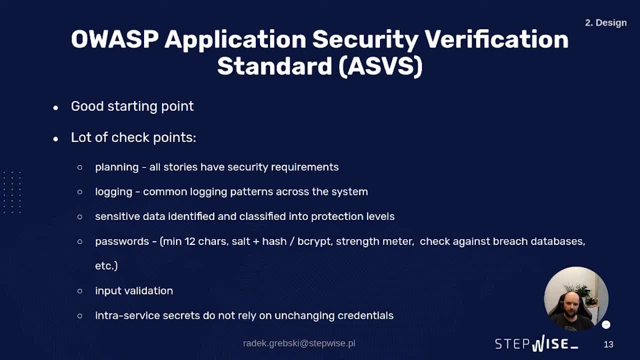 stories should also have security requirements. we should at when we log information, we should use common login patterns across the systems. we should identify the sensitive data and classify it into protection level, like i said before on on username or id number and ip address examples. we should define requirements for passwords. we should, of course, salt and hash passwords or we should use 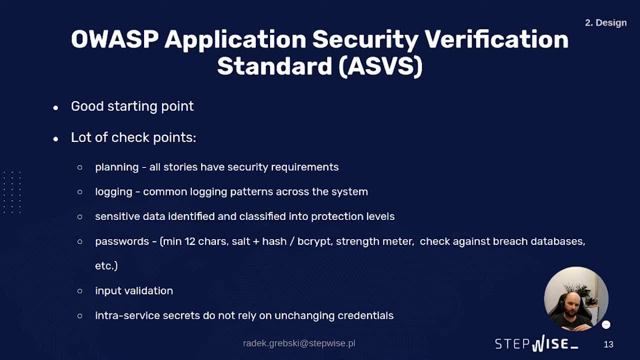 bcrypt. for that. we should use strength meter and triggervor and check against bridge databases of our password. We should do input validation. Intra service secrets, like passwords to the database, should not rely on changing credentials. And, as you can see, this is just like a six out of dozens of advices. 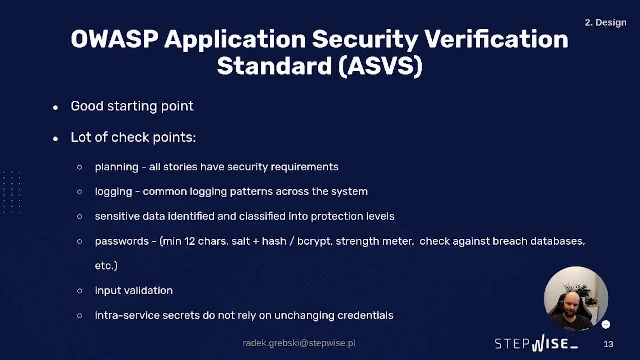 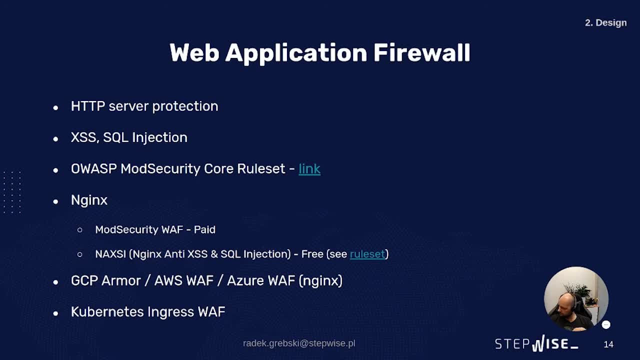 that you can take advantage of and you can implement it easily into your development process. There is also something called web application firewall, which gives you protection from most common HTTP attacks, which is cross-site scripting, as calling injections are generally the most often attacks. 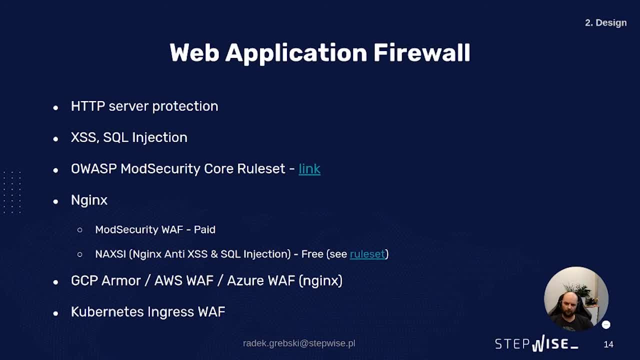 There is also open Ovasp also has model security core rule set where you can see the rules that web application firewall can use. Nginx has a mod security web application firewall. There is Nginx anti XSS and SQL injection. 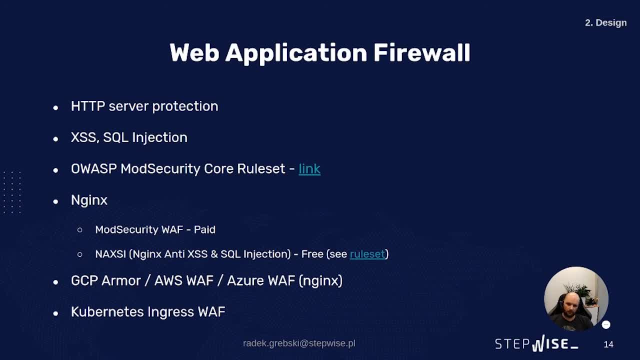 which is called Nuxie, And all cloud providers have their own WAF servers. for example, GCP has are more, AWS has WAF, wav and azure also have wav, which is based on nginx, and, of course, kubernetes ingresses also have their respective wav web application frameworks that you can use. okay, so we? 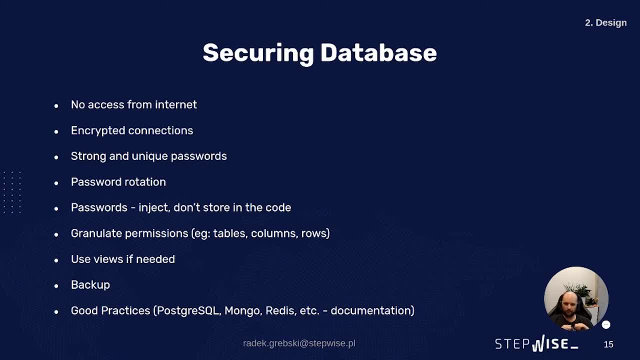 at the design. we also should think how we're gonna secure database or other external systems. uh, so we should. unless it's really really necessary, we shouldn't have access to our database from the internet. we should use encrypted connections, use strong and unique passwords and, of course, rotate them. that should be included in our policy. 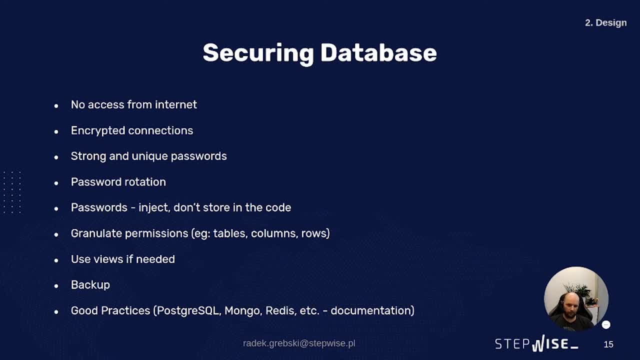 of course passwords should be injected. we shouldn't store them in a code, at least in, not in a plane text. we should granulate permissions. for example, if possible, we should add access only to tables, columns or rows, if it makes sense just to give minimal required permissions for each user. and if we cannot give an access to a table for a user, we can use views and 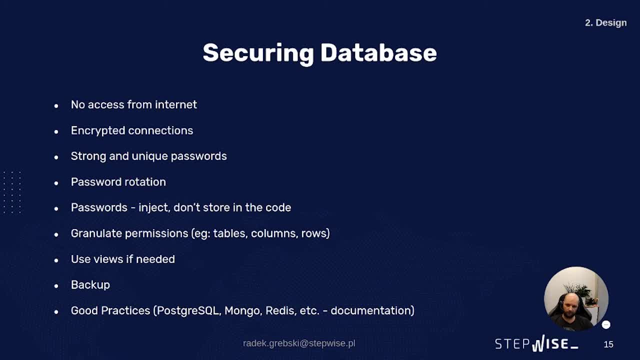 limit the data that is available in the database. as we see, everybody can use that as well. so please let us know in the comments if you have any questions or questions. you can ask us at the shown in on on a view, of course we should do backup of our database or any. 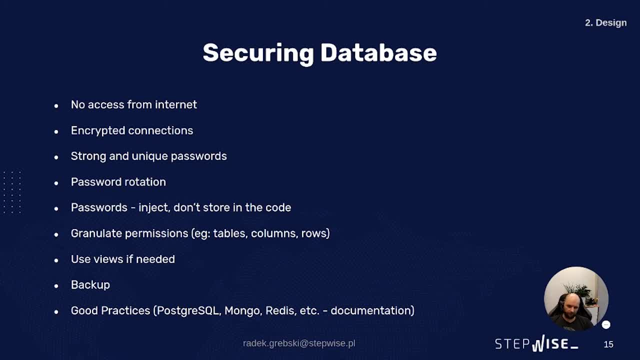 other external storage system. and, of course, when we do backup, we should in regular, on a regular basis, we should test the restore procedure, not only have backup. moreover, databases have their own good practices in documentation. so if you use, for example, Postgres, Mongo, Redis or anything else, check the.